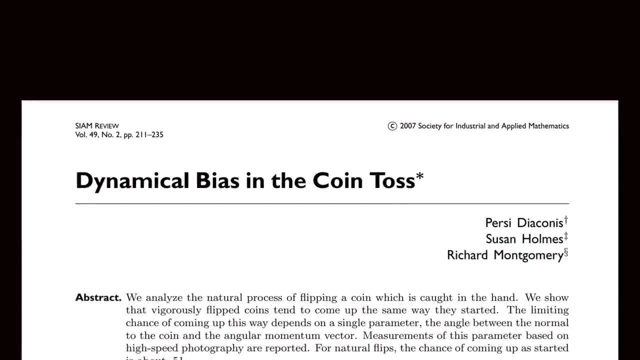 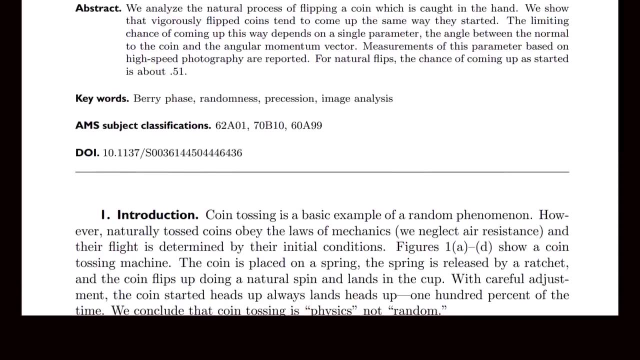 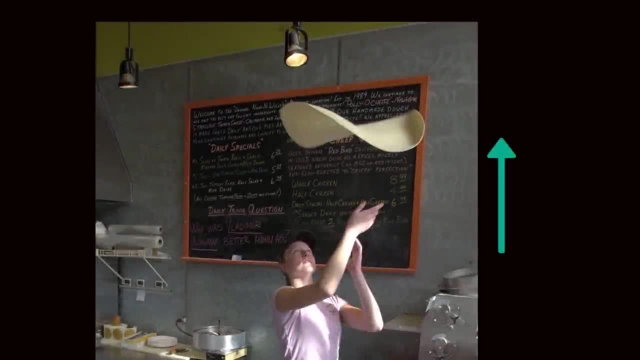 In 2007,, a paper by Diaconis Holmes Montgomery suggested the human mechanism of flipping a coin introduces a bias To understand it. think about hand-to-hand tossing a pizza dough. If you throw the dough up and it spins, it will land back on exactly the 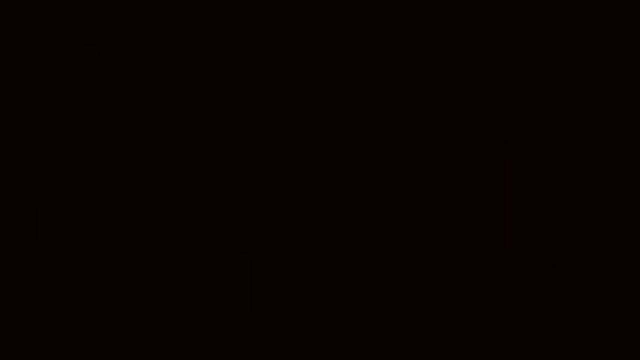 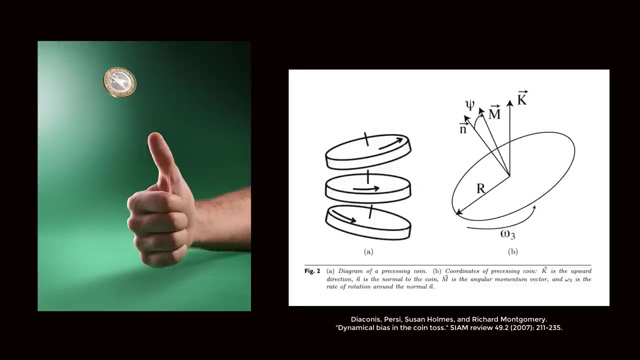 same side as it started. The same bias can happen when you toss a coin. When you try to toss a coin and flip it, you introduce a slight wobble in the spin, which makes the coin slightly more likely to land on the same side as it started. The mathematics and physics of why this happens. 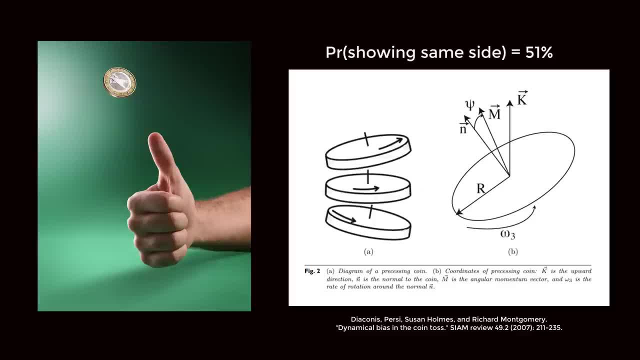 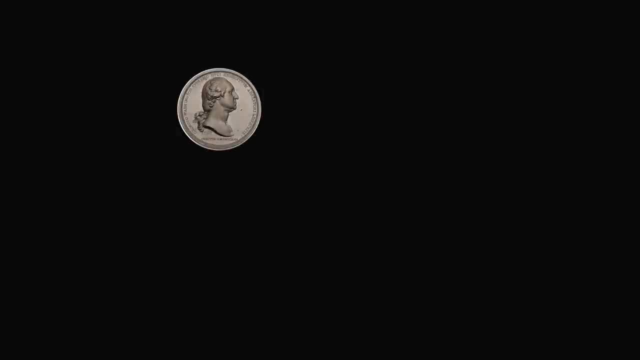 are trying to prove the same. If you toss a coin and it spins, it'll land back on the same side as it started. tremendously complex, But in the end they found a theoretical same-side bias of 51%. If a fair coin starts heads, it will end up as heads with a 51% chance. 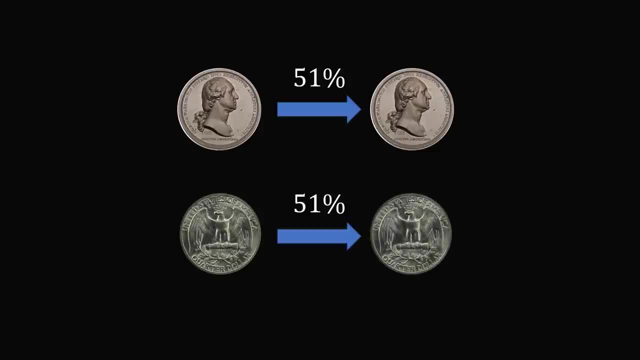 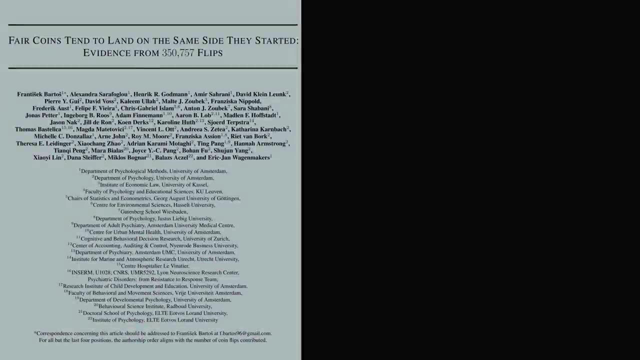 If it starts tails, it will end up tails also, with a 51% chance. But just how accurate is this theoretical model? A group of researchers just tested this out with one of the largest coin flipping experiments ever in history. A group of 48 people tossed coins of 46 different currencies and denominations and obtained 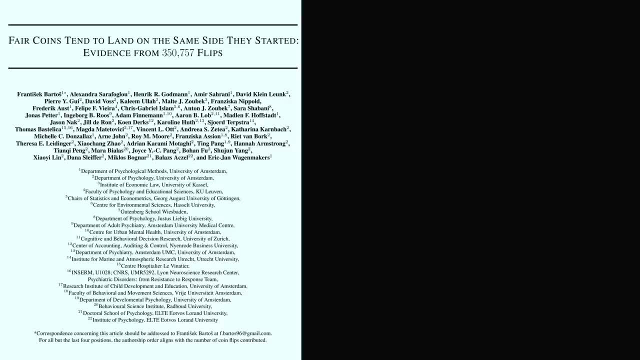 a total of 350,757 coin flips. In each sequence, people started with a random heads up or tails up position. They flipped the coin and caught it in their hands. Then they recorded the landing position. They then proceeded with the next flip and continued in a marathon of coin flipping. 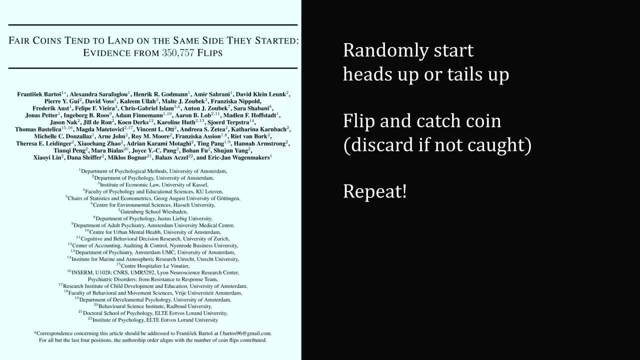 In case the coin was not caught in someone's hand, the flip was designated as a failure and they repeated the procedure. Out of all of this, they found a bias of 50.8% to land on the same side. But notice, the coins themselves were not biased.